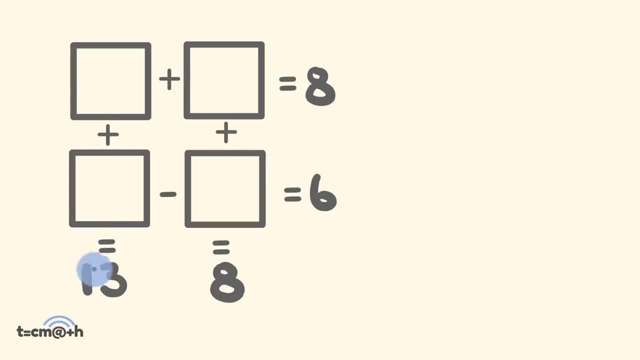 will be equal to 6.. This number plus this number will equal 13.. And this number plus this number will be equal to 8.. So pause this video if you'd like to give this problem a try, And when you're ready to keep watching and learn how to solve this problem, start up again. 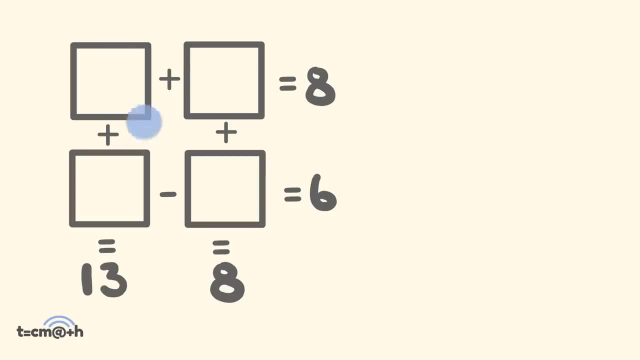 So how can we solve this problem? First off, let's label these four unknown numbers. to help us out, We'll call this one A, this one B, this one C and this one D. Now we know a couple of things here. 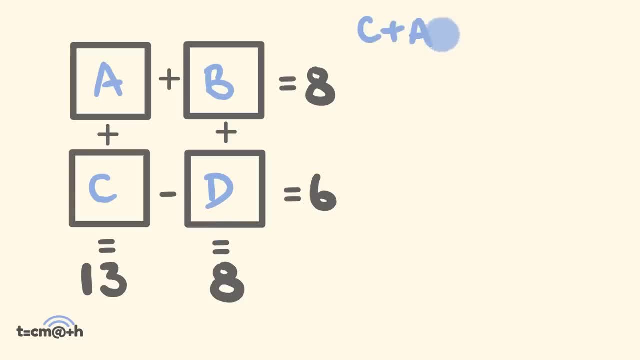 We know that C plus A is equal to 13.. We also know that B plus A is equal to 8.. So we can use elimination to form a new equation where A will cancel out A, A subtract A, C will subtract B, and here we'll have 13 subtract 8,. 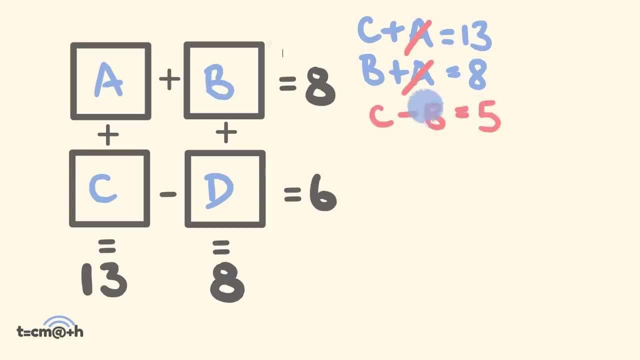 leaving us with 5.. So we have a new equation relating to C and B. We also know that B plus D is equal to 8.. We know that C subtract D is equal to 6.. So, once again, we can use elimination to form a new equation. 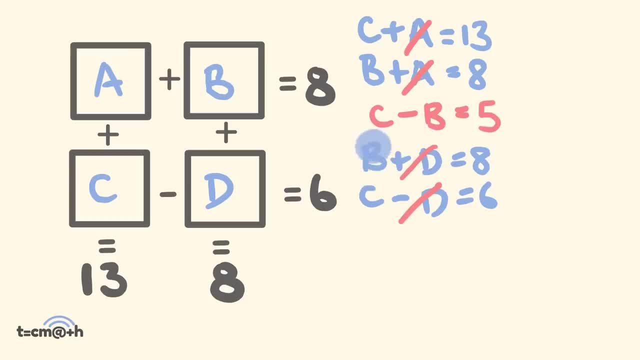 Positive D and negative D will cancel each other out. What we will do here is we will end up with C plus B, And on this side we'll have the product of 8 and 6, which is equal to 14.. Now we have two brand new equations relating to C and B We can use once again. 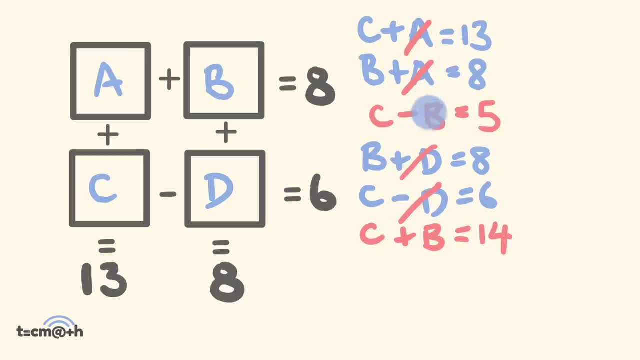 simultaneous equations to solve these. So, as you can see, negative B is equal to 14.. So we have two brand new equations relating to C and B. We can use, once again, simultaneous equations to solve these. So, as you can see, 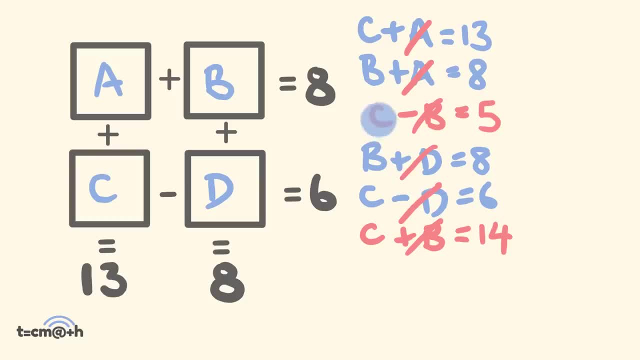 positive B and positive B cancel each other out. when we put these two equations together, C plus C is equal to 2C. This is equal to 14 plus 5,, which is equal to 19.. Therefore, what do we have? Well, if 2C is equal to 19,. C is equal to half of that, which is 9.5.. 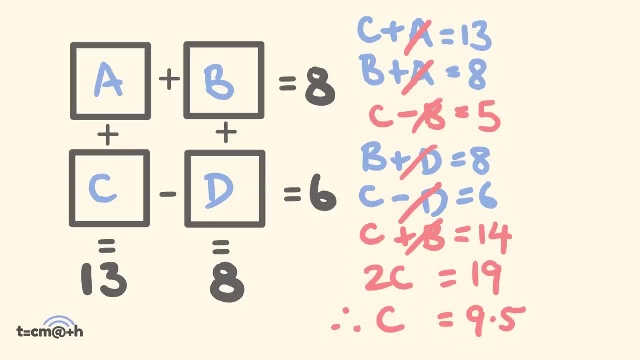 So we can go through now and start substituting in some values. We know that C here is equal to 9.5.. What else do we have? 9.5? take away what equals 6. This will be 3.5..